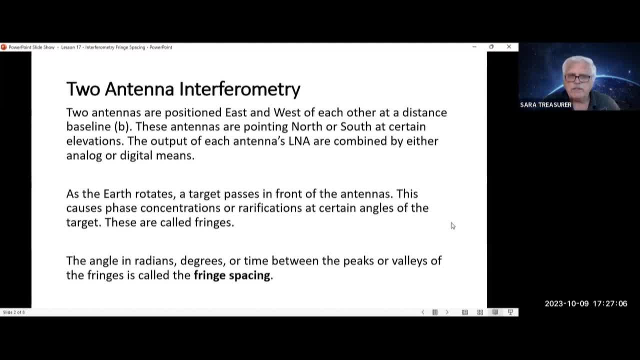 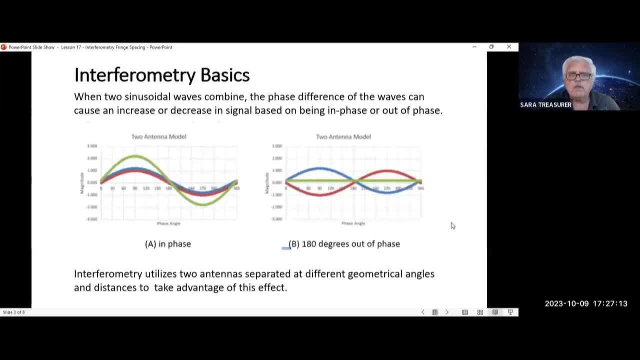 These are called fringes. The angle and radiance degrees are timed between the peaks or valleys of the antenna. The fringes are called the fringe spacing. Some basics: When two sinusoidal waves combine, the phase difference of the waves can cause an increase or decrease in signal based on being in or out of phase. 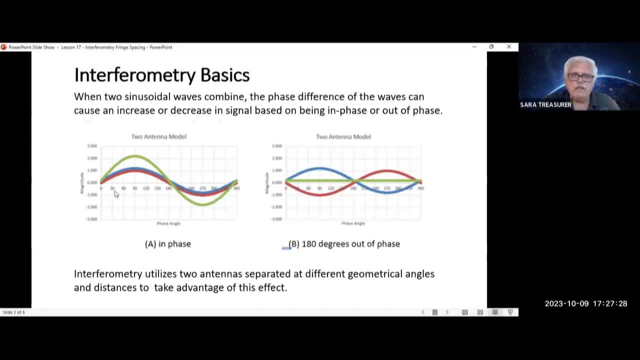 You see diagram A. You see that two signals, the red and the blue, are in phase. The resulting additive signal is higher. The initial two signals are higher than the initial two initial signals. If these are 180 degrees out of phase, they look like this: The red and the blue. 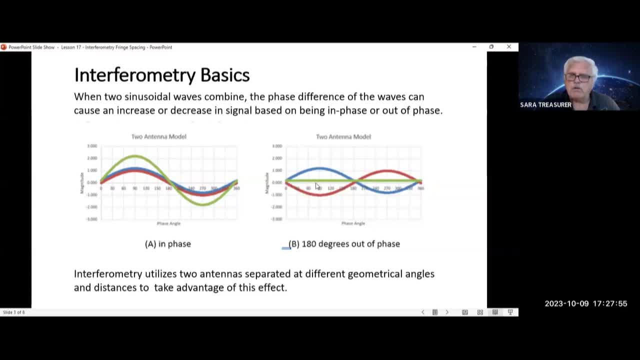 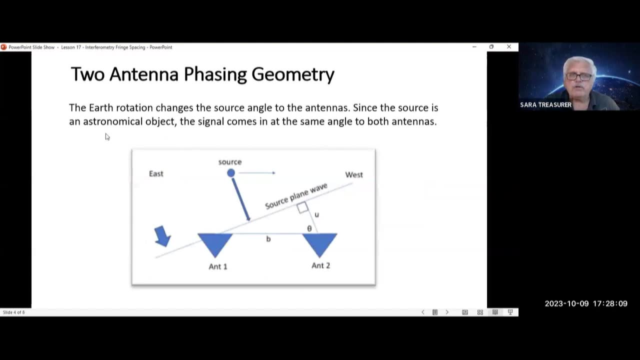 And the final added output is zero. So interferometry utilizes two antennas separated at different geometrical angles and distances to take advantage of this effect. During drift scanning, the Earth rotates. During drift scanning, the Earth rotates. The Earth rotates changes the source angle of the antennas. 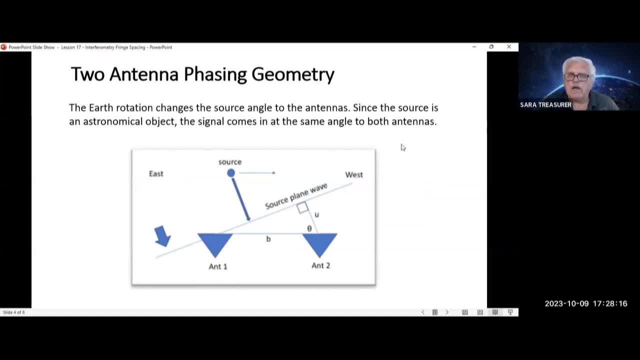 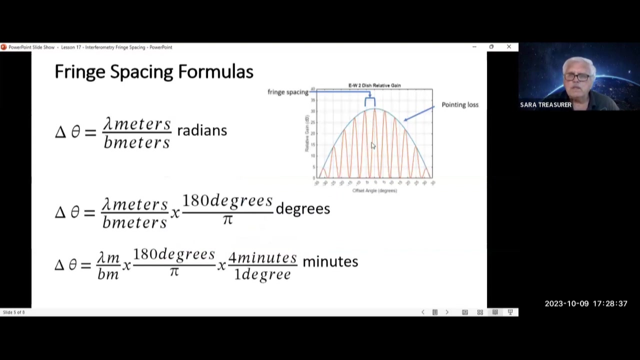 Since the source is an astronomical unit object, the signal comes in at the same angle of both antennas. The distance between the antennas is B, The angle is theta. Let's look at the formulas. If you look at, If you look at, If you look at. 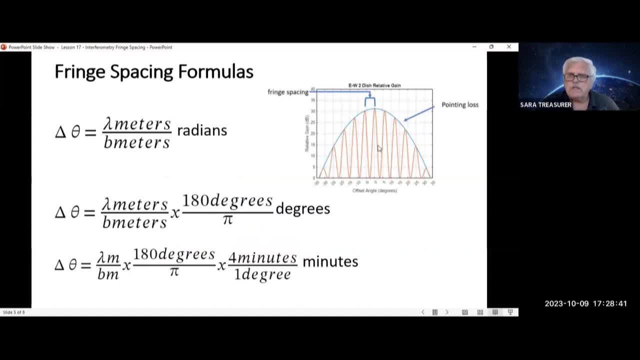 a common drift scan. you see how the fringes come up and down and you see the peaks. The distance between the peaks is the fringe spacing. We'll call that delta theta To get radians. delta theta is equal to the wavelength over the distance B. 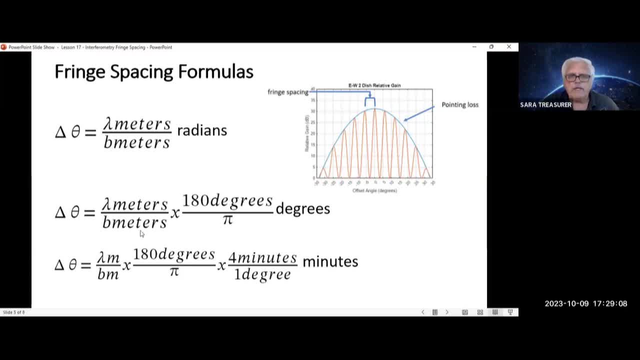 I'll give you radians. To convert the radians to degrees, you multiply that answer by 180 degrees over pi And, when you're drift scanning, figure out how many minutes in between each of these peak fringes. You multiply that answer in degrees times four minutes per one degree and that'll give you the answer in minutes. 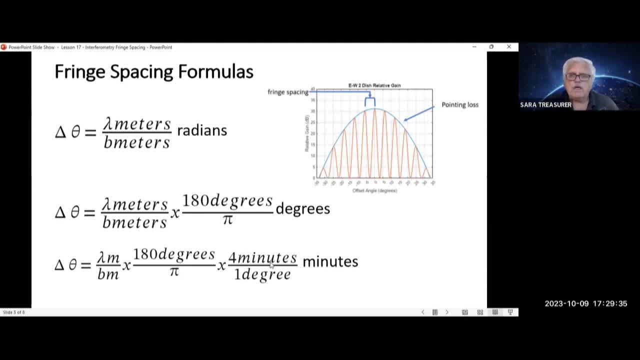 You multiply that answer in degrees times four minutes per one degree, and that'll give you the answer in minutes. And note that the four minutes over one degree is how fast the Earth rotates during a drift scan. And note that the four minutes over one degree is how fast the Earth rotates during a drift scan. 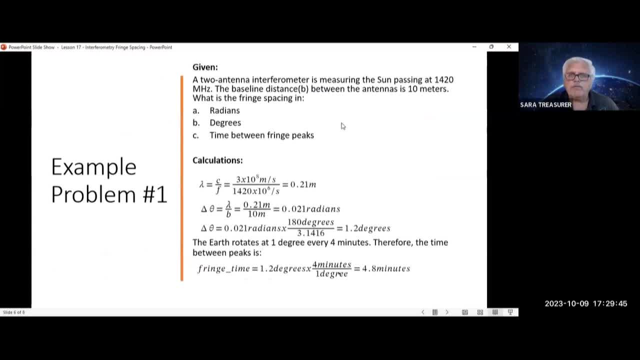 Let's do an example. You have a two-antennas interferometer and you're measuring the Sun at 1420 megahertz With a baseline distance B between the antennas of 10 meters. what is the fringe spacing in radians, degrees and time between fringe peaks? 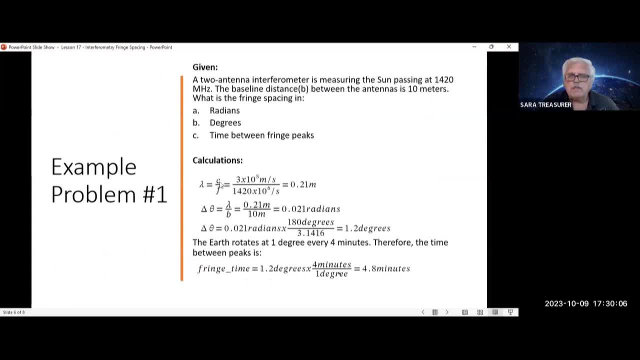 So first you calculate the wavelength That gives you the speed of light over frequency. That's 3 times 10 to the 8th meters per second. Over 1420 times 10 to the 6th per second is equal to 0.21 meters. 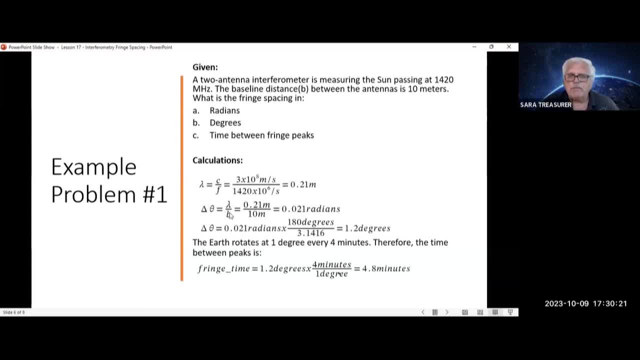 Fringe spacing in radians is equal to your lambda over B. 0.21 over 10 gives you 0.021 radians. Converting that to degrees, you take that answer Times 180 degrees over pi 3.1416.. 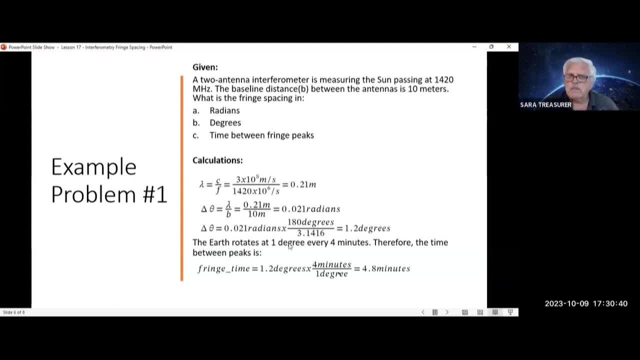 That will give you 1.2 degrees And, as we said during drift scans, the Earth is rotating at 1 degree every four minutes. Therefore, to convert the 1.2 degrees to minutes, you take that times 4 minutes over 1 degree is equal to 4.8 minutes. 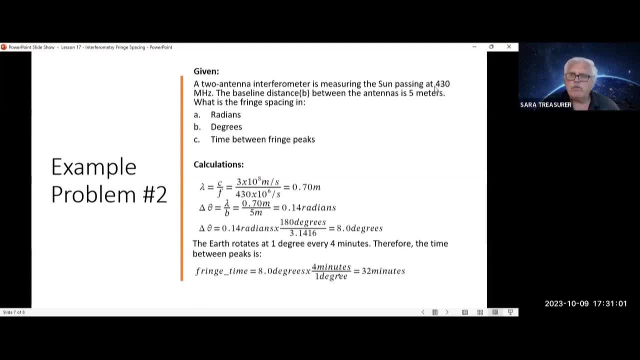 Let's do another example. This time we're going to use 430.. 430 megahertz with a distance of 5 meters. Calculating the wavelength, that will give you 3 times 10 to the 8th meters per second. 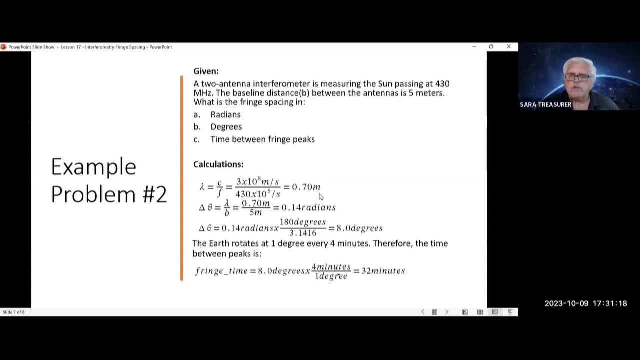 over 430 times 10 to the 6th per second is equal to 0.70 meters. Fringe spacing in radians is your lambda over B. It's equal to 0.7 meters over 5 meters And that will give you 0.14 radians. 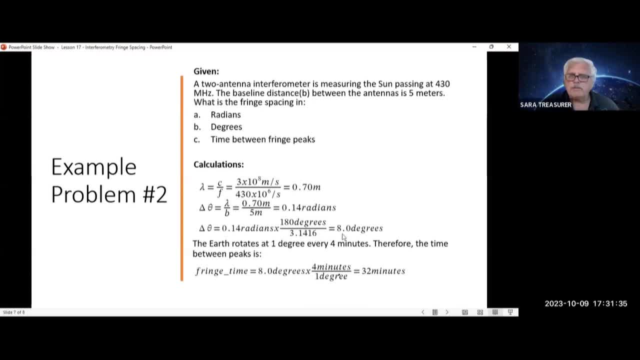 Converting that to degrees, you multiply that times 180 over pi, It's equal to 8 degrees. And converting that to minutes with a drift scan, that will give you 8 degrees times 4 minutes over 1 degree is equal to 32 minutes. between all those peaks.